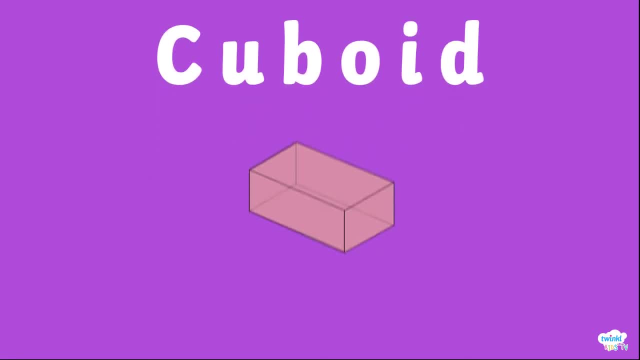 A cuboid is a 3D shape. It has 6 faces. This shape also has 12 flat edges. A cuboid has 8 vertices. You will find that a cereal box is the shape of a cuboid. Next up is the cone. 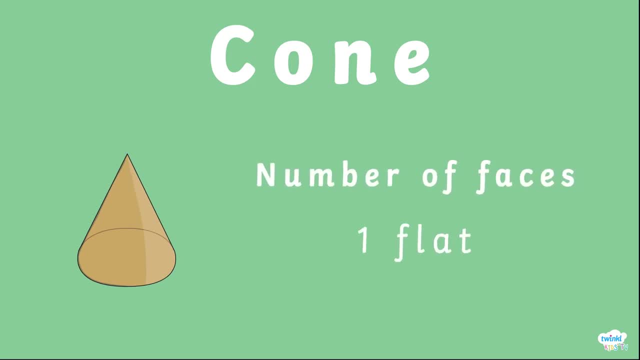 It has 1 flat face. A cone also has 1 curved face. The number of edges a cone has is 1 and it is curved. An ice cream cone is an example of a cone. A cylinder is another 3D shape. 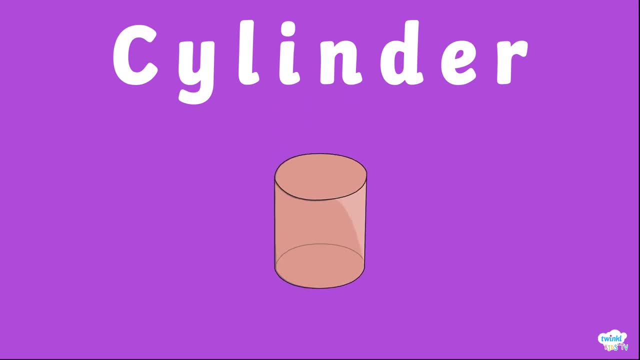 A cylinder is another 3D shape. This shape has 2 flat faces, One at the top and one at the bottom, and one curved face around the shape. This shape has 2 curved edges. A baked bean tin or another type of tin is a cylinder. 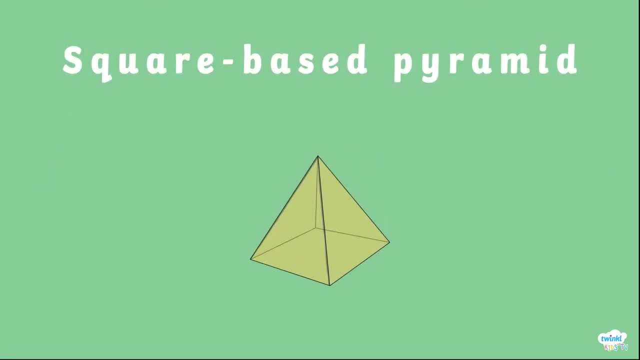 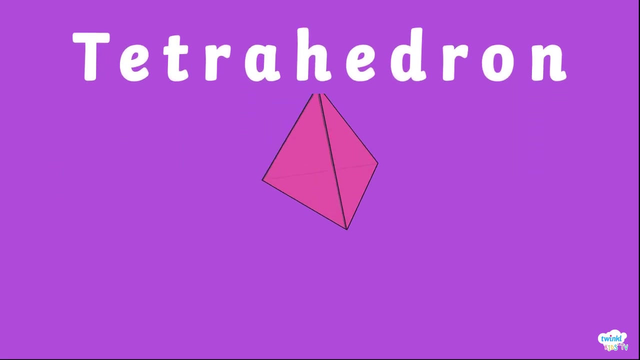 A square based pyramid is next. This shape has 5 flat faces. It has 8 flat edges. The number of vertices this shape has is 5.. You can find a square based pyramid in Egypt. A tetrahedron is similar to the square based pyramid. 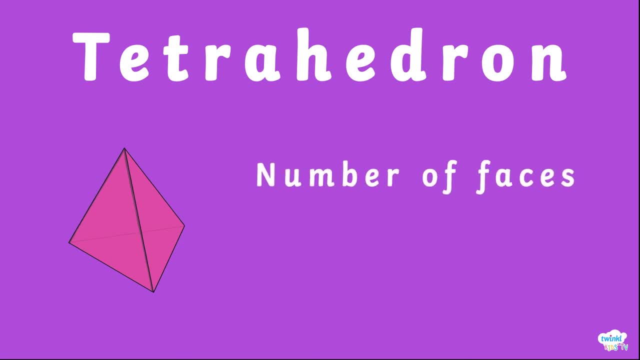 But it has a triangular base. This shape has 4 flat faces. The number of edges it has is 6 flat. The number of edges it has is 6 flat. This shape also has 4 vertices. An example of a tetrahedron is a triangular dice.